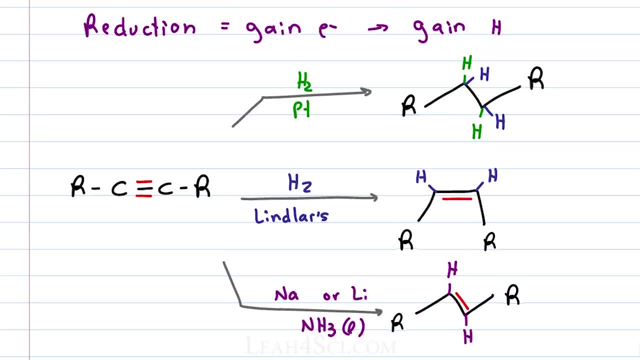 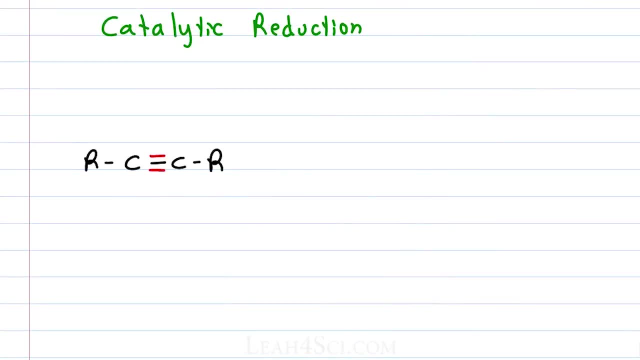 from each other for a trans product. Let's go into each reaction in more detail. Catalytic reduction of alkynes is very similar to what you saw from alkenes. Recall from alkene reactions that catalytic reduction takes an H2 gas and puts it onto the pi bond. 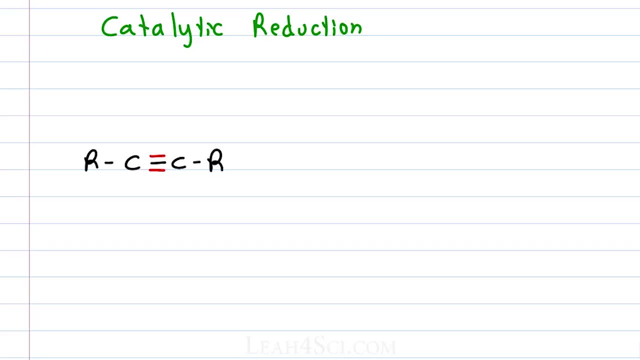 and breaks the pi bond, adding to the same phase of the molecule. The mechanism isn't fully understood, but we have some idea as to what's going on. Imagine that you have a metal catalyst that is holding hydrogen atoms. This is because the H2 gas already 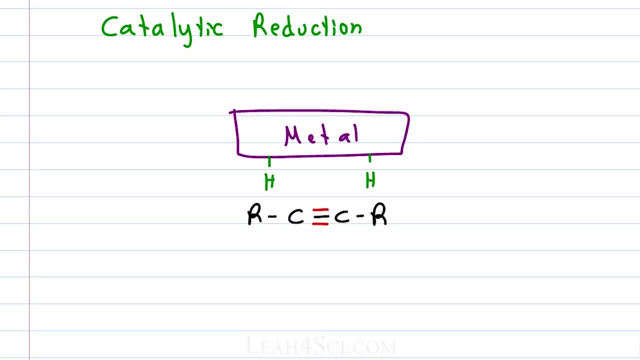 broke apart and was grabbed by the metal and is just sitting on the surface of the metal. Now imagine that the metal is going to reach for the carbon atoms and when it does so, it breaks that pi bond between them. This is why the reaction is a sin addition, because the metal grabbing the carbon reaches 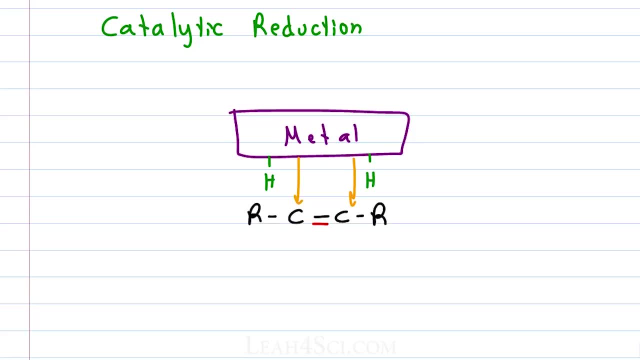 for both carbons at the same time, from the same position, and then the hydrogen atoms that are also sitting on the metal will simply slide over and attach onto the carbon atoms They're adding from the same phase of the molecule. This would happen to both phases of the pi bond, so that your ultimate product is a carbon. 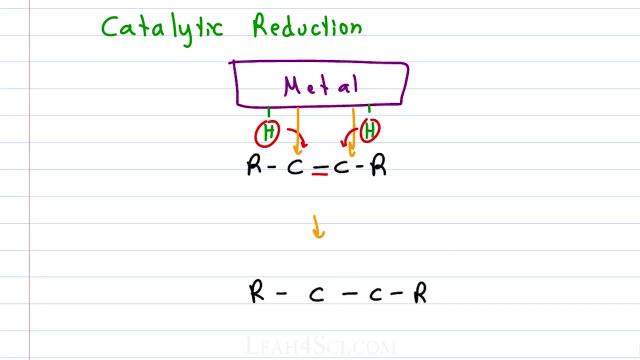 chain with just a sigma bond between the two carbons and then two sets of hydrogen atoms having added together at the same phase. So we'll show green for the first pi bond that we broke and blue for the second. This is a fully reduced alkane. 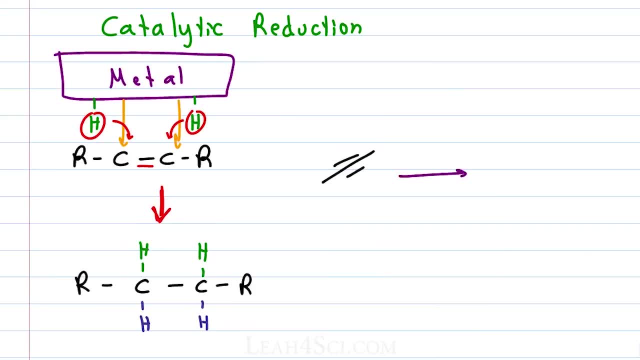 When you write out this reaction, you have to specify or assume that it's H2 in excess, because to reduce an alkyne with two pi bonds we're adding two sets of hydrogen atoms. You'll see it shown with the word excess, just the letters XS, or even two molar or two. 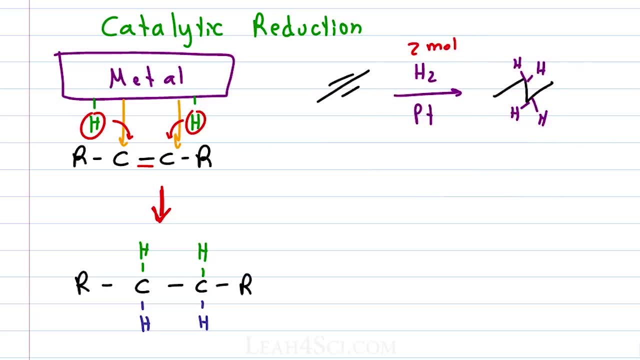 equivalents to show that we're adding two moles. But don't think that two moles means if I decide to only put one mole, then we'll only have one pi bond broken. that's not the case, Because imagine the situation where you start with three alkynes and you're thinking: if 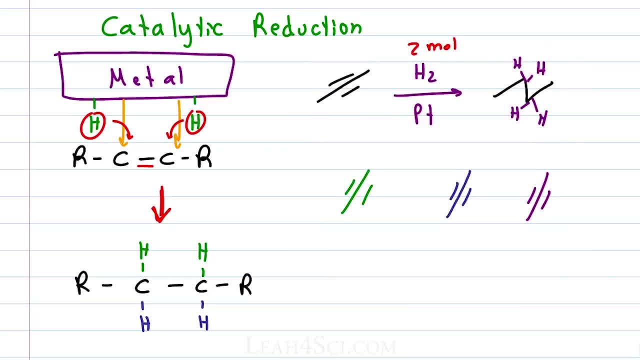 I only use three moles of H2 gas, Then each alkyne is going to break. Each alkyne will have one H2 added and I will get an alkene product. That is not the case, because it's not easy to control and the product will be random. 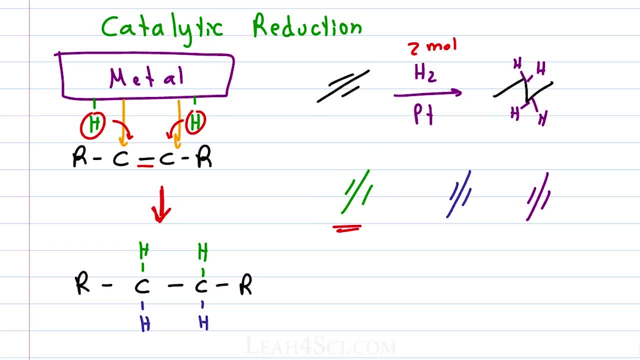 The green one might get zero reduction, giving you an alkyne as your final product. The blue one might get a double reduction, giving you an alkane as your final product, and the purple one might go halfway, giving you an alkene product. This is not all alkene. it's nothing complete. 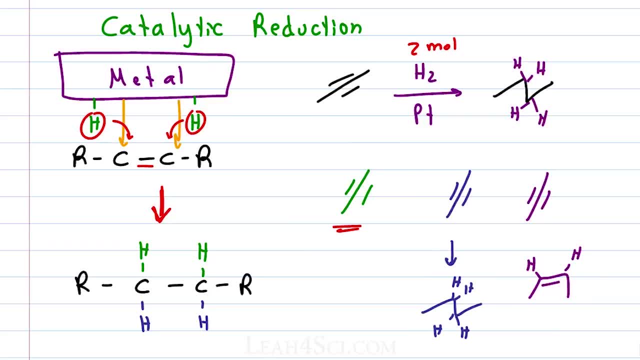 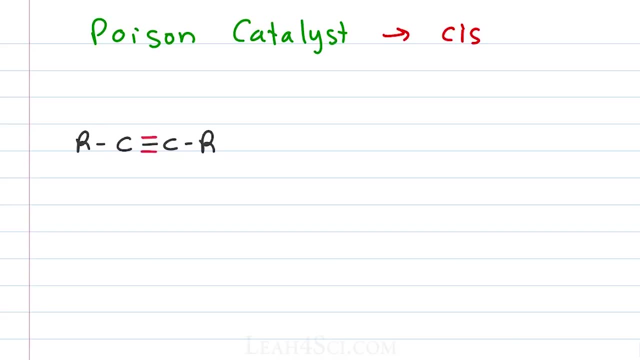 Complete and partial, Definitely not effective to get a product. So what do you do if you want a catalytic reduction that stops at the alkene? Question is: do you want cis or trans? In order to get a cis alkene, we have to use a poison metal catalyst. 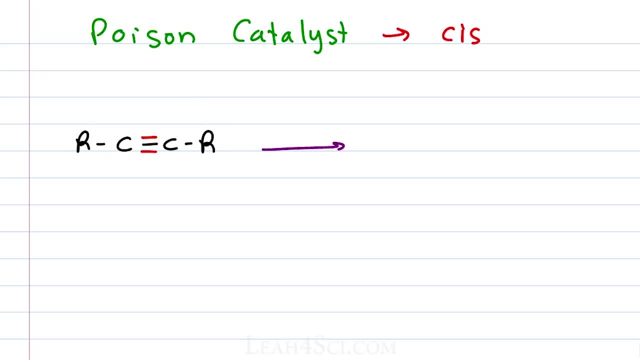 A poison metal catalyst still uses H2 gas. That means we're still adding the hydrogen, but being that the catalyst is poison, it's a little slower, It's a little effective And it's only capable of adding one rather than two moles of H2.. 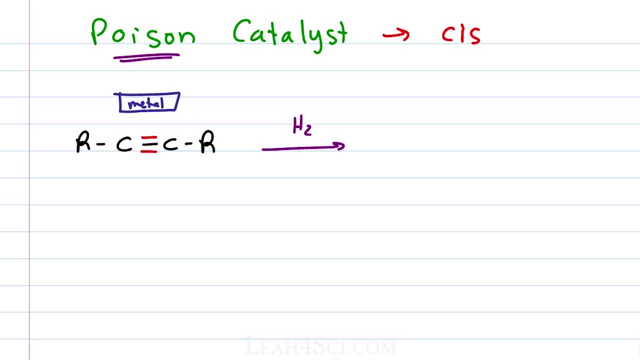 Imagine that the metal, as sluggish as it is, works the same way. It grabs the carbon from the same face and adds the two hydrogen atoms to the same face, Showing this with one pi bond still intact and the two hydrogen atoms having added to. 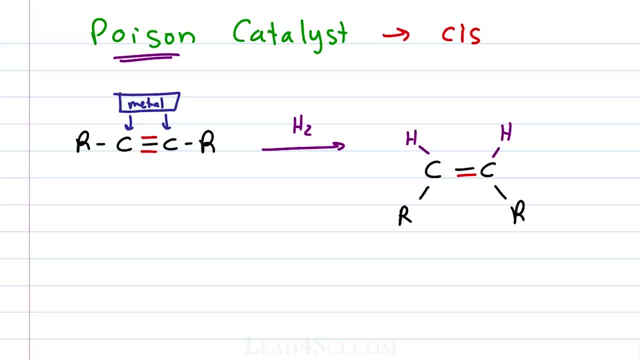 the same face. the two R groups get pushed down, get pushed away for a cis product. The most common poison metal catalyst that you're going to see in organic chemistry is the Lindler's catalyst, and I like to think of it as the lazy catalyst. 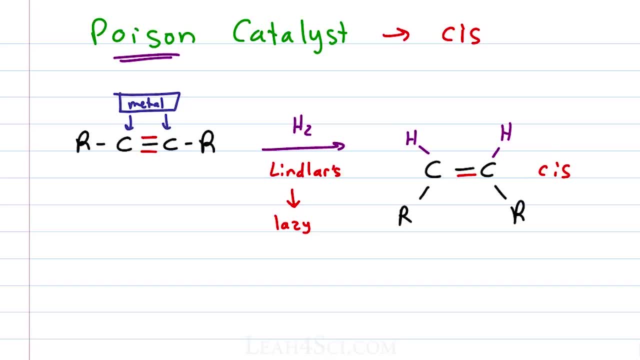 It's so lazy it does half a job and then it quits. Most of you will only have to recognize Lindler's without the details, but in case your professor asks, the Lindler's catalyst is a monstrosity that looks like this quinoline palladium. 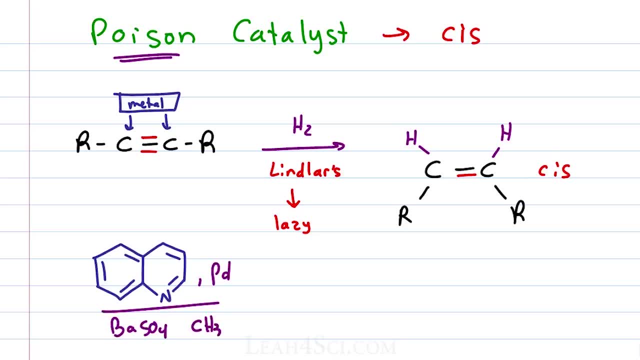 dissolved with barium sulfate in a methanol solution. Okay, Or we could just say Lindler's, much easier. Don't memorize Lindler's cis, understand why? So the key why in this reaction is that a metal grabs from the same face: the hydrogens. 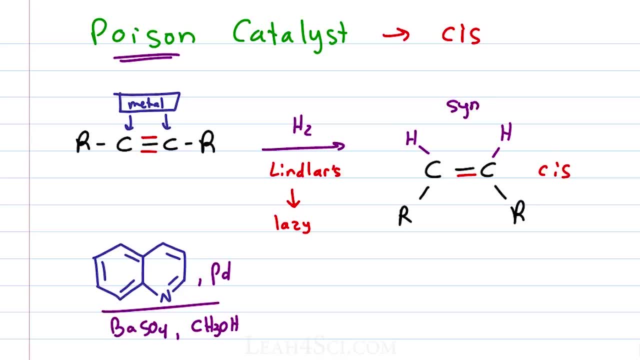 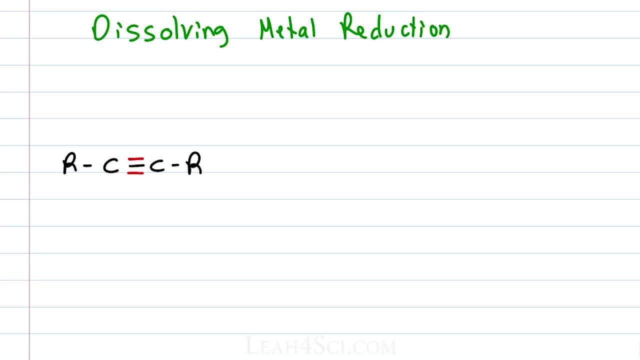 get added syn to each other and that gives us a cis product. This is opposite of the dissolving metal reduction, where the key intermediate that determines the why is a radical Okay And that radical intermediate will force a trans final product. This reaction happens because we're using a group, one element which, in its neutral state, 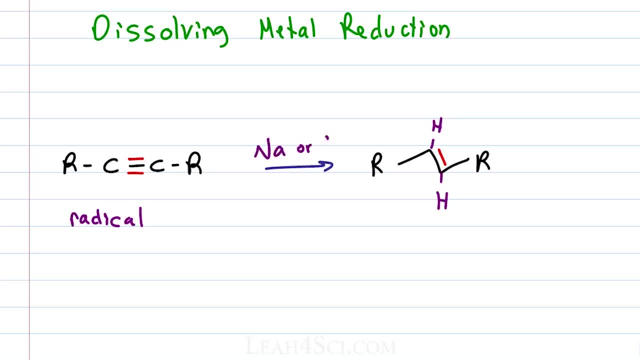 has just one valence, electron, For example sodium or lithium. This is dissolved in a cold solution. ammonia at room temperature is not liquid, but if it's really cold it will be liquid with a radical intermediate. Let's take a look at the mechanism. 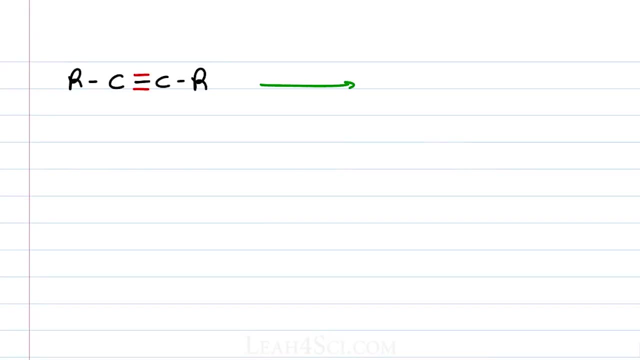 So you understand exactly Why it goes trans. This mechanism starts out with a sodium in solution. even though it's neutral, it should be happy. it's not. It has that one unpaired valence electron, making it very unhappy and it doesn't want. 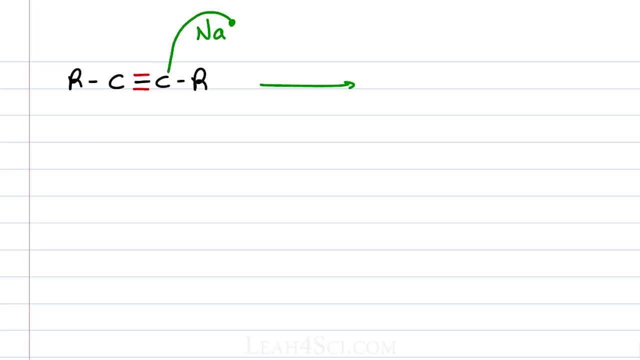 the electron, so it gives it away and it gives that electron to the carbon atom. Notice we're showing the mechanism with a single headed or fish hook arrow to represent the movement of one rather than two electrons, Making this a radical mechanism. I also want you to follow the colors of every electron as we move along, so you understand. 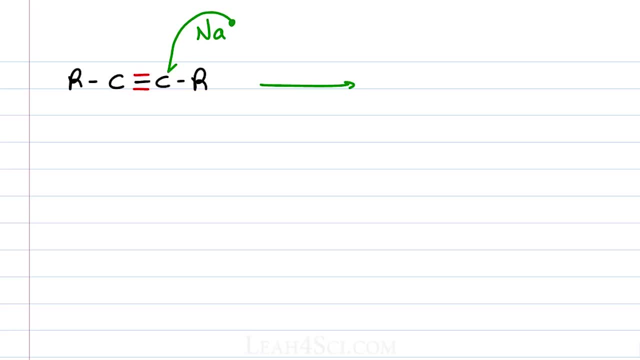 exactly where things are moving and why they're doing what they do. We'll show the pi bond as two red electrons breaking apart When carbon gets that. one green electron from sodium. that electron does not want to be by itself. So one electron from the pi bond with a fish hook arrow showing that just one electron. 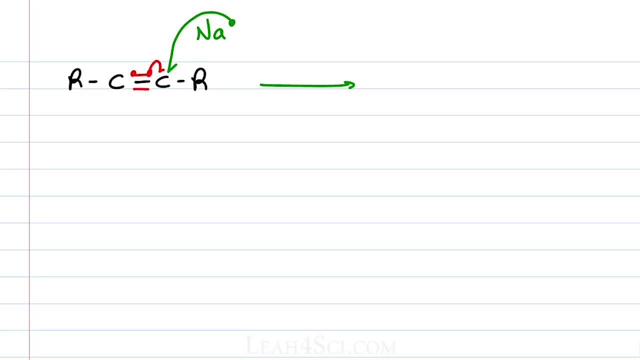 moves over to meet that green electron and form a lone pair. Okay, The other electron gets kicked away. It's a third wheel, there's nothing for it, and so it breaks away onto that second carbon. Our intermediate looks something like this: On the right, we have a green and a red electron with a lone pair and therefore a negative. 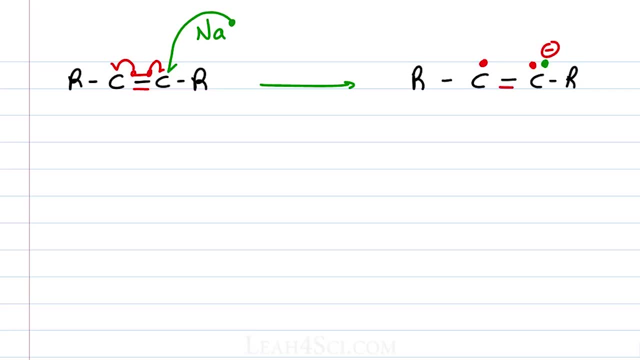 charge. On the left we have a neutral radical. This, right here, is where we determine that the product will ultimately be trans Soon. as we go from the triple bond, which is linear, To the double bond, the angle changes. We have two options. 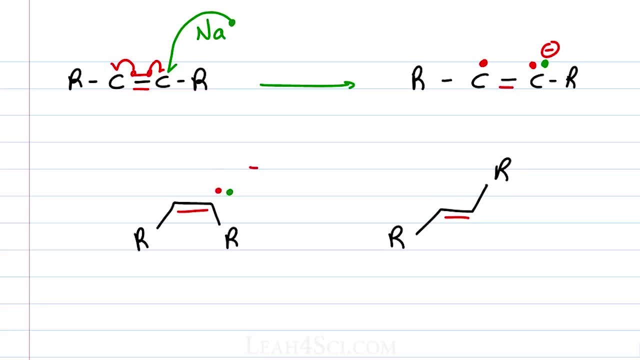 On the left, we'll show the lone pair of electrons cis to the radical. On the right, we'll show the lone pair of electrons trans to the radical. Don't forget, These electrons have their personal space and the VSEPR theory. valence shell electron. 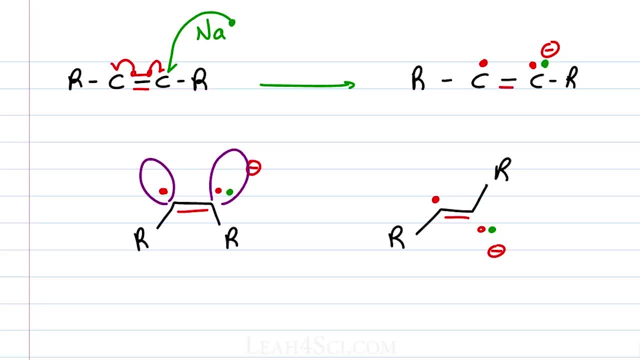 pair repulsion tells us that they don't like being next to each other. When we have this cis intermediate, the two electron clouds are too close together. Electrons near electrons makes them very unhappy, very unstable and therefore not likely to form. On the right, we have the two electron clouds as far away from each other as possible. 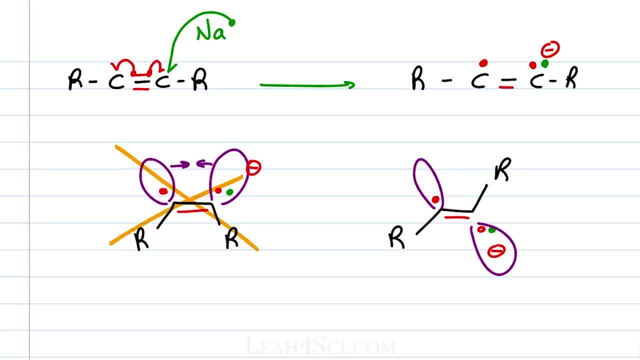 Having the lone pair of electrons facing completely, anti, completely away from that radical. They're as far away from each other as possible, making this the absolute most stable intermediate. And since the molecule had to adopt a trans configuration, the ultimate product will also be a trans configuration because of this intermediate. right here, 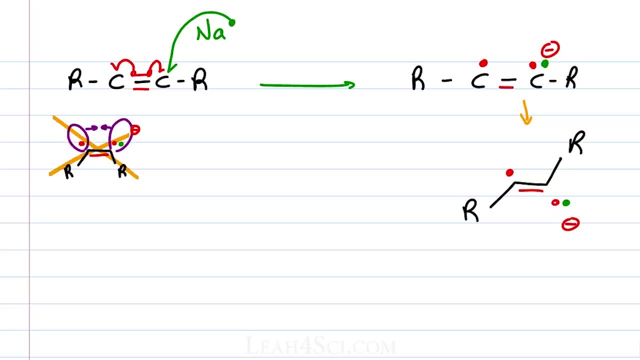 But we have too many electrons going on and this is very unhappy. Remember this reaction takes place in NH3 liquid, which means we have ammonia floating around everywhere. Ammonia is a polar protic solvent With a partially negative nitrogen atom And a partially positive hydrogen. 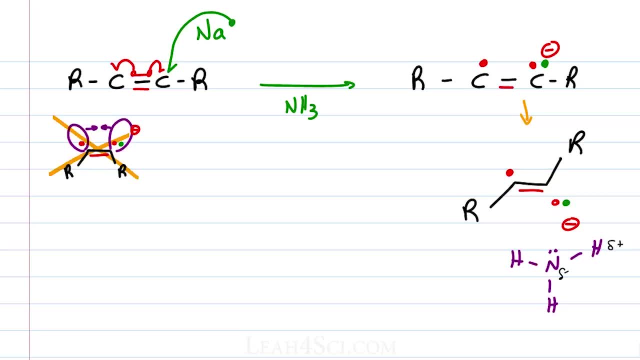 That partially positive hydrogen will attract the lone electron pair, The one that's made from the green and red electrons. These electrons will reach out for one of the hydrogen atoms, breaking the bond between hydrogen and nitrogen, to collapse those electrons back onto the nitrogen atom. 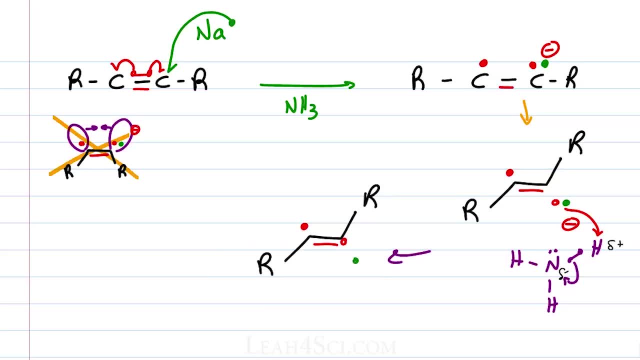 The green and the red electron are still attached to the molecule, but now they're sitting as a bond between carbon and the purple hydrogen we grabbed And the purple hydrogen we grabbed from ammonia. We also have an NH2 remaining in solution with a lone pair of electrons from the initial. 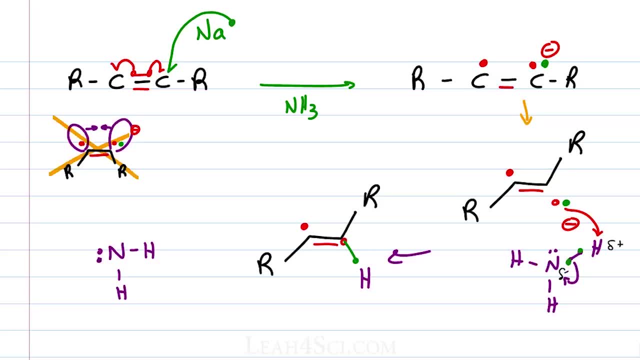 nitrogen and a second lone pair from the bond between hydrogen and nitrogen that collapsed, giving this a negative charge. Well, guess what? That's sodium. When it donated its electron, gave us an Na plus, and this is now a positive, negative ion. This gives us a balanced sodium.